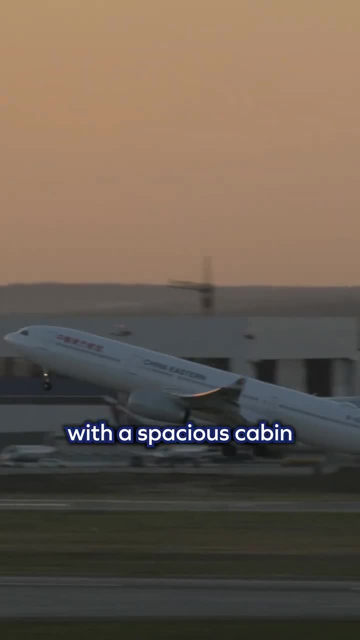 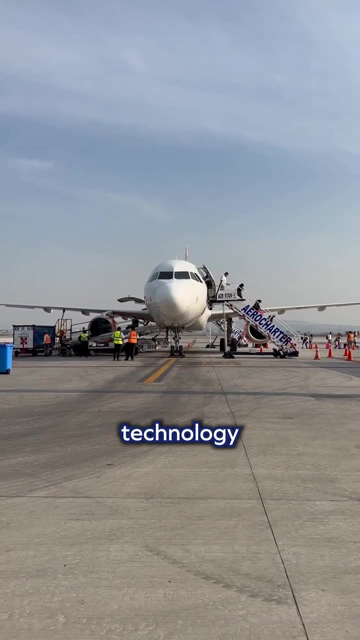 the A330 is a versatile, long-haul twin-engine jet with a spacious cabin and impressive range. The big brother to that is the A350, Airbus's modern wide-body jet featuring advanced materials and cutting-edge technology. And then behold the massive A380, the world's largest passenger jet. 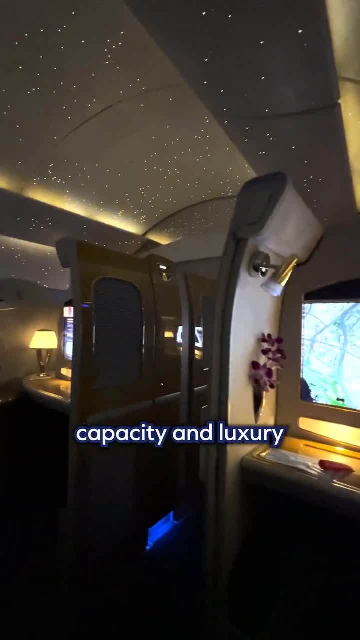 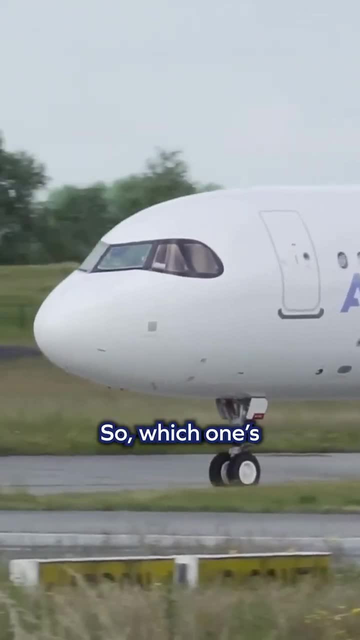 a double-decker wide-body aircraft offering unparalleled capacity and luxury. Finally, the A321XLR, an up-and-coming narrowbody, ultra-fuel-efficient jet, perfect for those lower-capacity long-haul routes. So which one's your favorite? 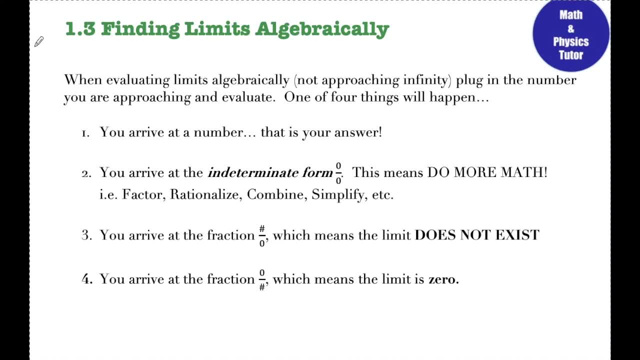 Hi everyone. today we're going to be talking about finding limits algebraically. So when I evaluate a limit algebraically, I'm always first going to plug the number that I'm approaching for my limit in for whatever variable I'm looking at, and just solve and see what I get. When I do that, 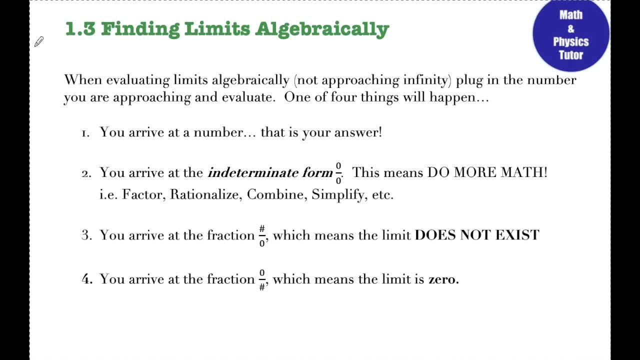 one of four things will happen that will determine if I need to do any more work or what my answer is. So the first thing that happens is I plug in my numbers and I get an answer. Perfect, I get a number over a number. There's my answer. I'm good to go. The second thing that can happen is once 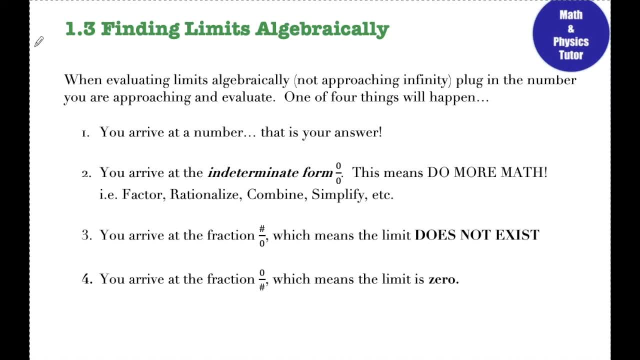 I've plugged in my numbers and evaluated, I end up with zero over zero. This is an indeterminate form and means that I need to do more math. That means that I need to either factor, rationalize, combine, simplify etc. Something to change what that expression looks like and then re-evaluate. 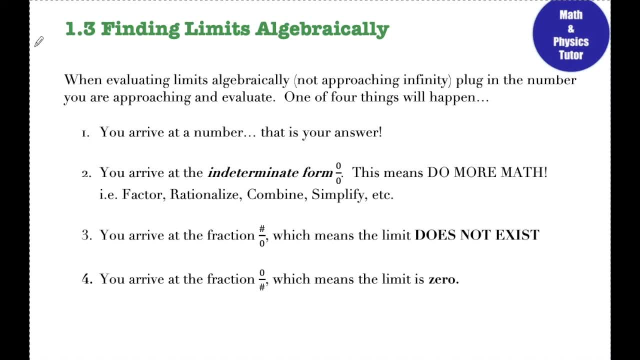 that limit again. The third thing that can happen is, once I've plugged in my numbers, I end up with a number over zero, Five over zero, Eight over zero, Whatever Something, number over zero. This means that the limit does not exist. That's a DNE limit. The fourth thing that can happen: once